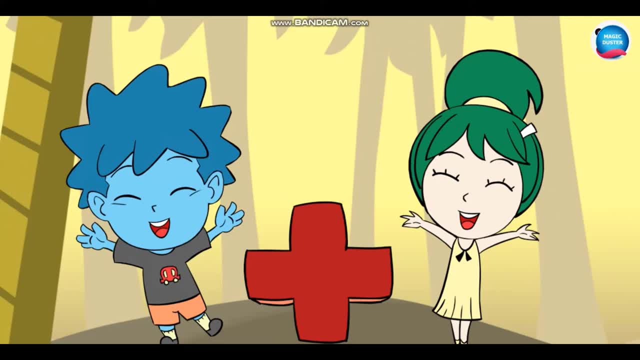 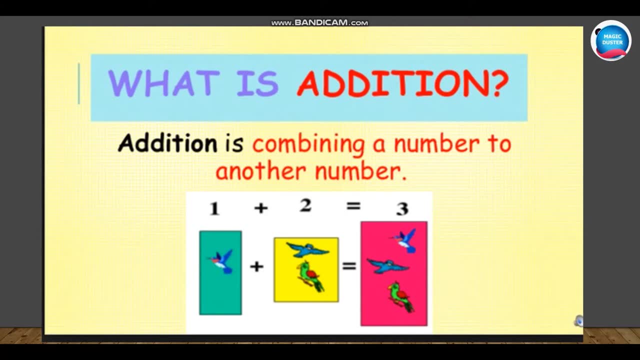 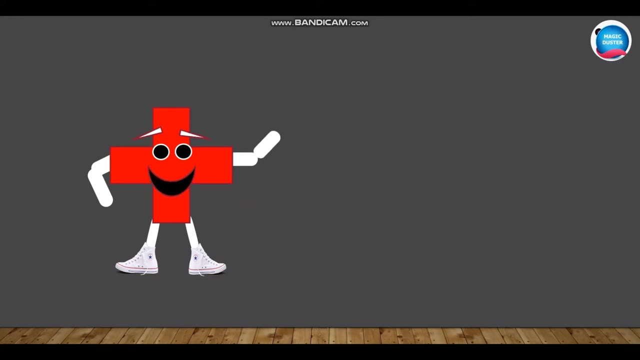 Yes, this is addition, which means the symbol of addition, And we know that addition is combining a number to the another number. Let us see in detail. Hi kids, I am addition, People used to call me plus. My duty is combining the number and. 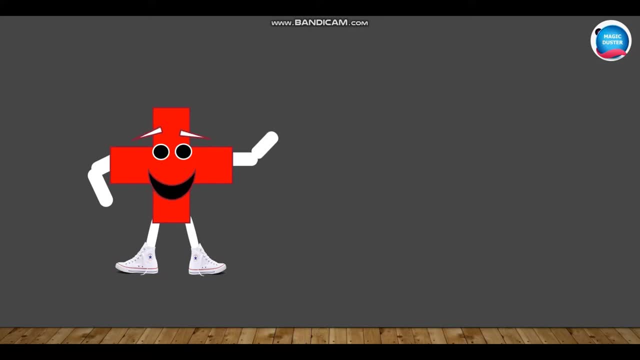 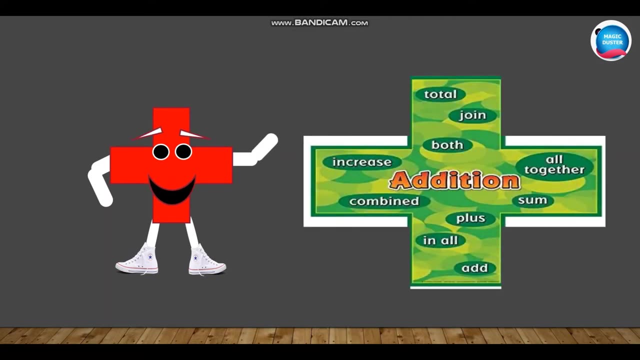 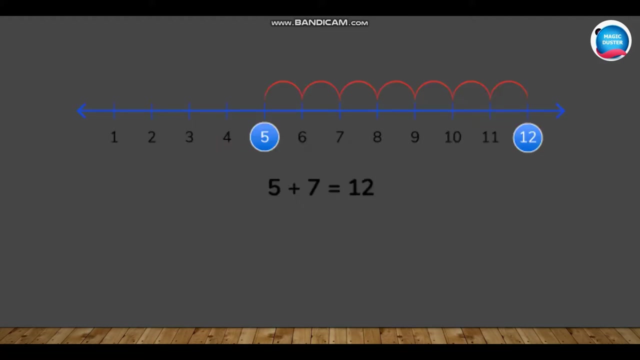 finding the total. Of course I have the pet names, just like you, That are total in all. sum in all together: Yes, children. So addition is easy to do. Let us see that. how to do the addition in number line. Here we have a sum 5 plus 7.. To find: 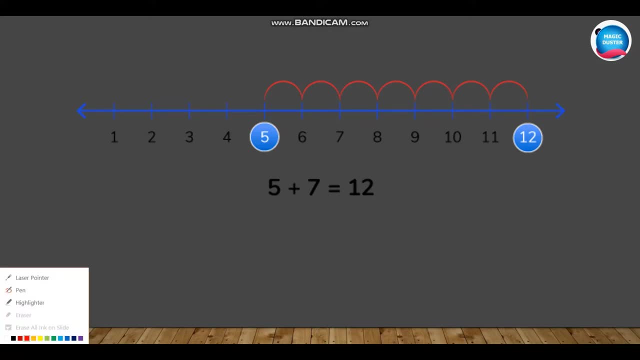 out the answer, I should start with the first number, 5.. I marked 5 and to find the total or to find the more numbers, we should go forward. so if i count forward, i should go for seven. next numbers: so it must be six, seven, eight, nine, ten, eleven, twelve. so what is my answer? 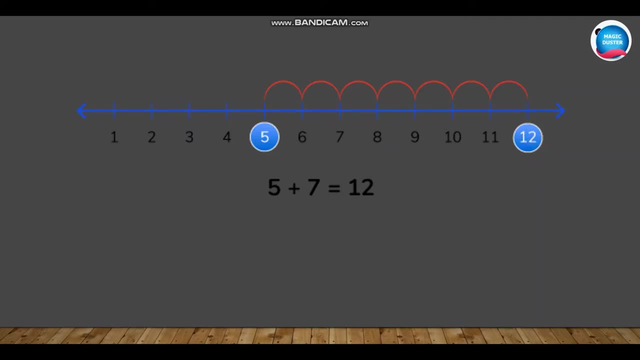 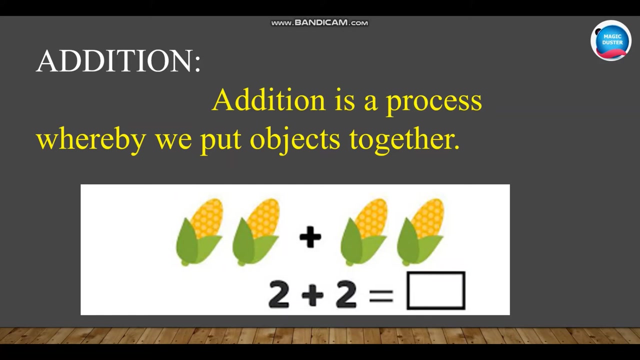 twelve. maybe if we are doing subtraction we have to count in a reverse order. to put that simply, addition is a process whereby we put objects together. here i have cons to count the cons. i can do addition two plus two totally. how many cons i have? four instead of cons, let us 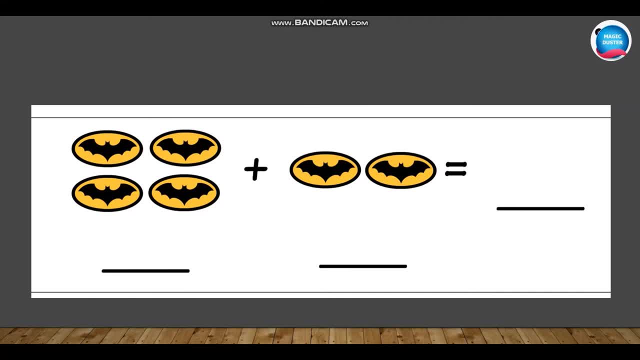 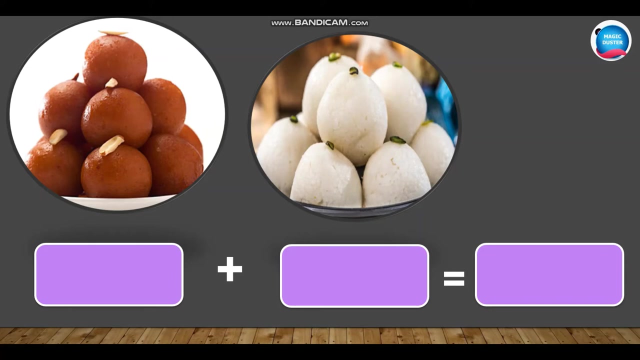 uh, let us add the stickers. i have batman stickers, so four, and my sister have two batman sticker, so two. if i add both the stickers, how many stickers? totally, we both have six. very good, let us learn one more example for this: there are 22 gulab jamuns on the table. 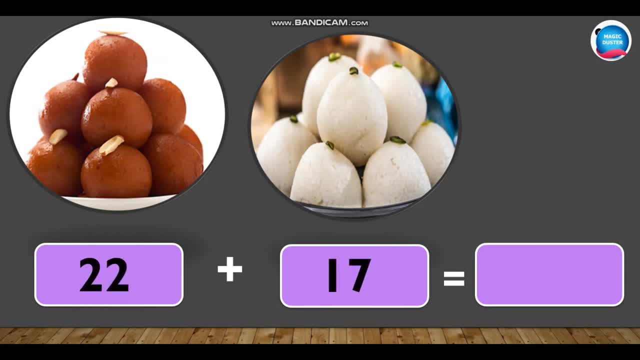 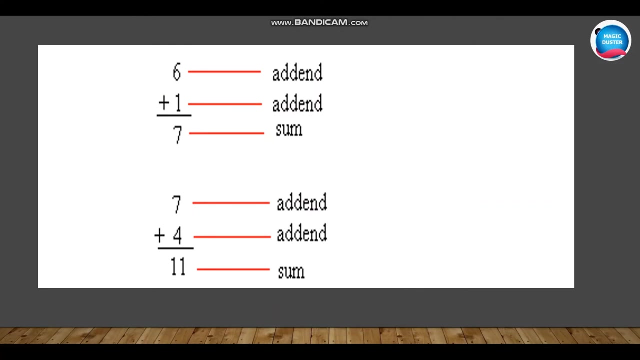 and 17 rasagullas also on the table. now, how many sweets are there in total? yes, 39 sweets are there in a total. so we are doing addition. always the answer must be the biggest one and, in addition, the things which we have to remember is addend and the sum. so to explain clearly the terms which we used in 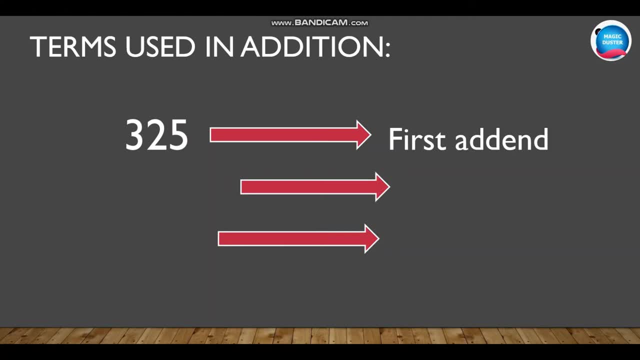 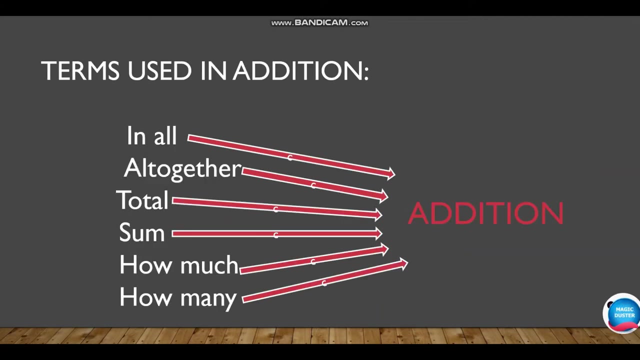 addition is first number, is first addend and the second one which we add up to is second addend and the answer is called the sum and, as i said before, the addition have so many pet names, so in max we can say that is terms. so what are the terms used in addition? in all, all together, total sum. 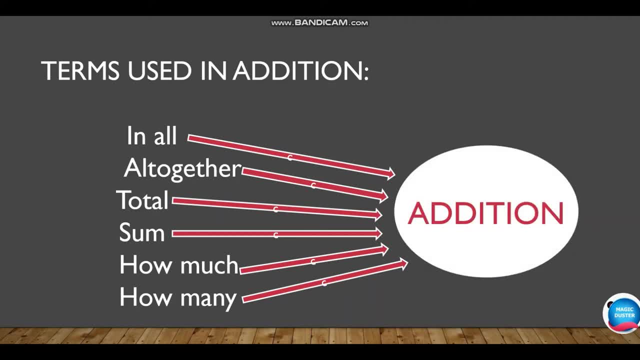 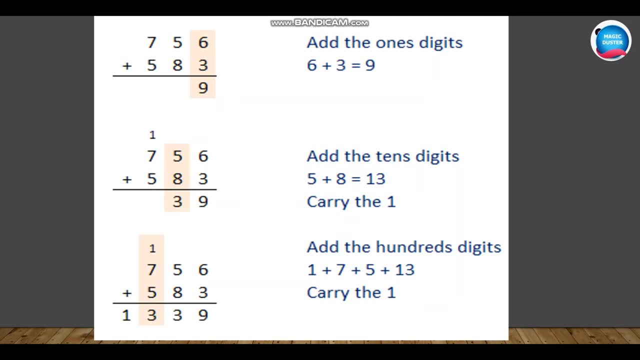 how much and how many. so these words are representing addition. here i have a sum. let us see how to do it: 756 is add up to 583. so to do the addition always we have to start with the ones column. not only for addition. for all the operations of max we should start with the ones column. 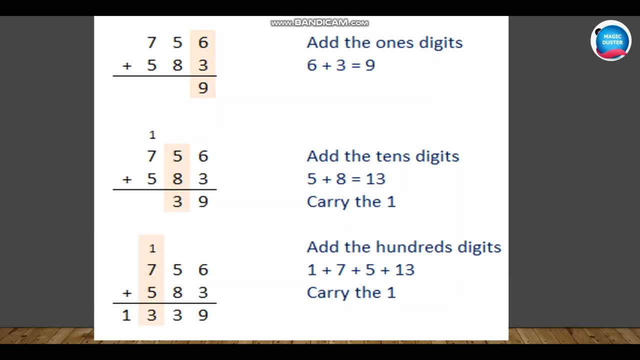 now 6 plus 3 is 9. i finish the ones column so i can go for the tens column. in the tens column i have 5 plus 8. if i add both the numbers, how many numbers? i received 13, but in one column i can write only one number, so i should write 3. 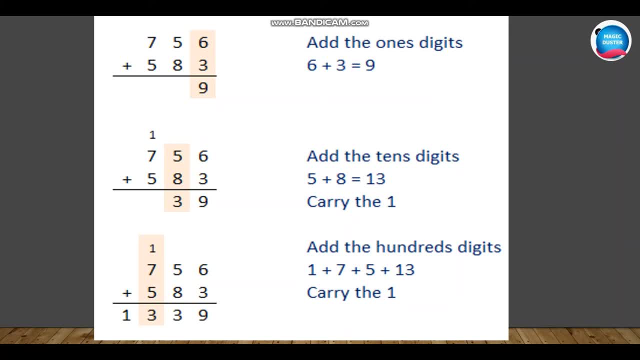 here and the remaining number should jump on the next neighbor head. so what is that hundred? so we should not call that number now 1. that is our carryover. let us jump into the hundreds, column seven plus five. so if i add these two number i got 12. 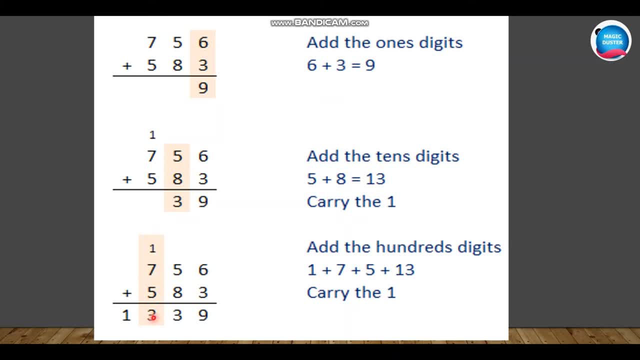 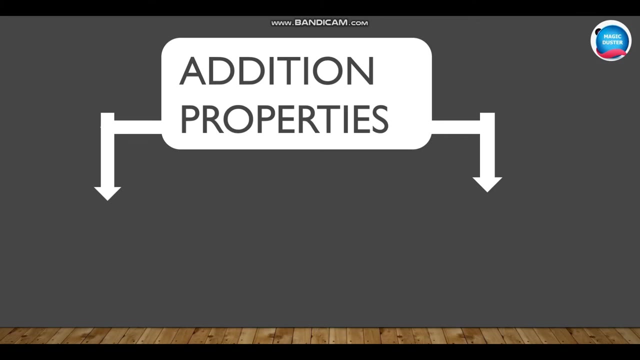 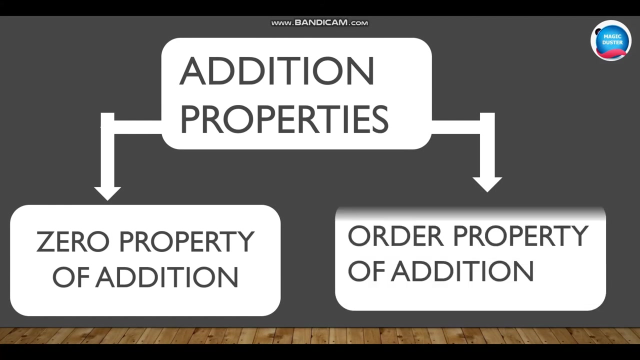 don't forget to add the carry over. so 12 plus 1 is 13. so what is my answer? 1339 is the answer. moreover, we have two properties and addition. so the habits of addition. let us see what was that. the first property is zero property and the second one is order property: zero property of addition. 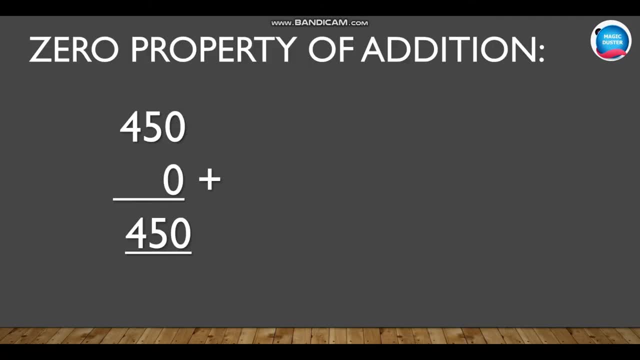 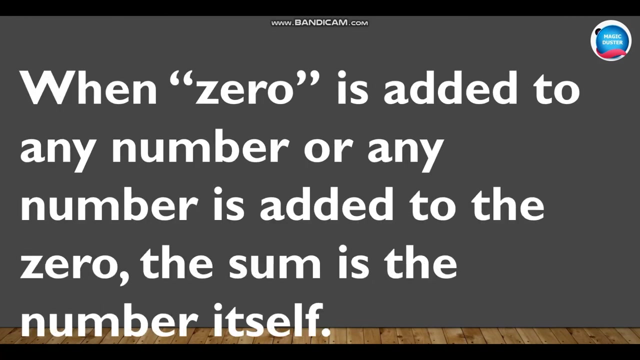 if i add any number to zero, i will receive the same number as answer. for example, 450 plus 0 is 450 and 22 plus 0 is 22. so when 0 is added to any number or any number is added to 0, the sum is the number itself.